to do with our matrix. we can always find our unknown variable values, even if our constant matrix changes. Well, if we think about what we want to do with our matrix, we can also find our unknown variable values, even if our constant matrix changes. 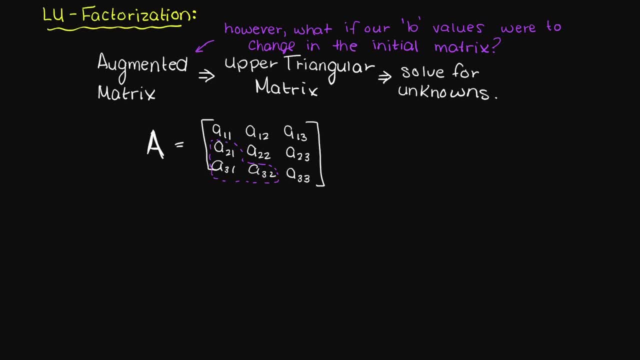 Now we know what we did during Gauss elimination. we solely focused on eliminating the purple region of our A matrix. Therefore, if we track what we do to our A matrix, we can easily apply that to our new B values. But how do we go about this? Well, we do this by placing 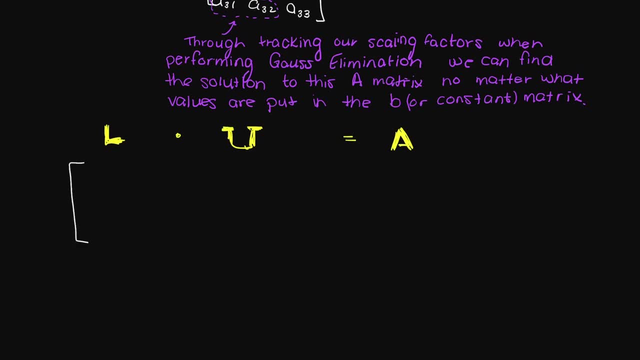 our scaling factors that we used in Gauss elimination into a lower triangular matrix. This is where the L? U and L? U factorization comes from. We have a lower triangular tracking scaling factors used to transform our augmented matrix into an upper triangular matrix. So in LU factorization we are creating two triangular matrices that, when multiplied, 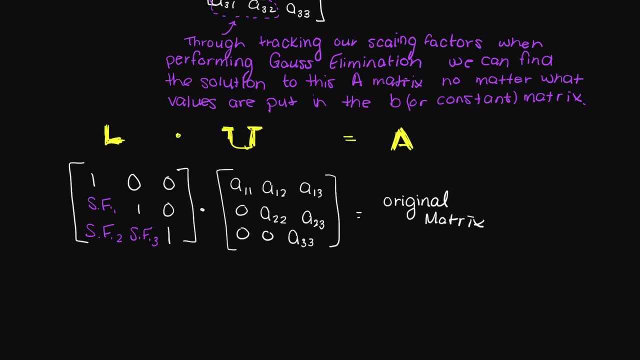 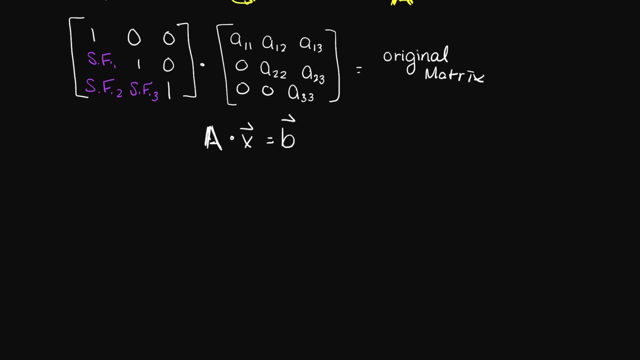 together give our original matrix. So let's quickly show how this works. We begin with our original matrix form: matrix A times our variable vector equals to our constant vector. Then, after performing our Gauss elimination, we are left with an upper triangular matrix. 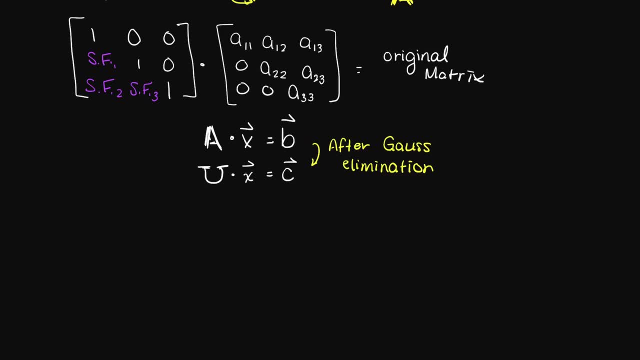 times our variable vector, which is equal to our new constant vector, since we must apply all the same changes here that we did in each row of our matrix, Now let's multiply both sides of this equation by our lower triangular matrix, which I will 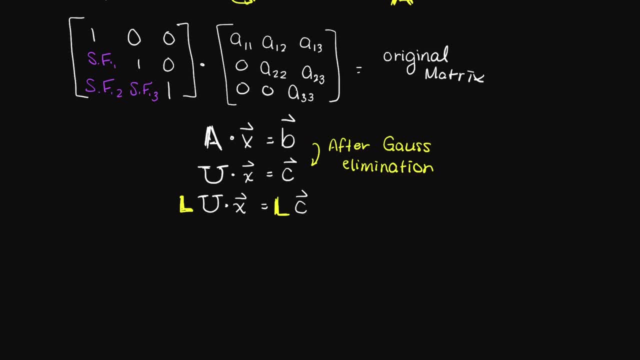 focus on more here shortly. Now we note that the matrix U times our vector variable is simply our new constant vector. therefore we are left with the following: This allows us to easily use our matrix L and our original constant vector. Then, using our newly solved constant vector times, our U matrix, we can easily solve for: 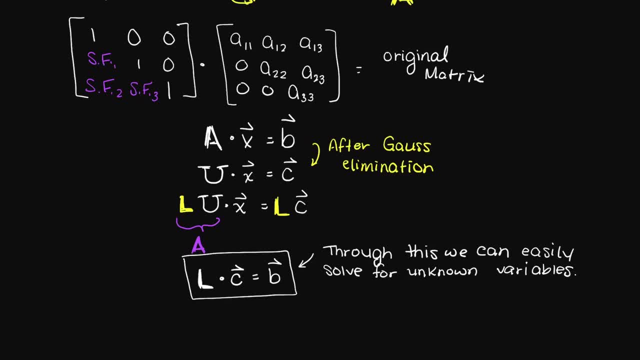 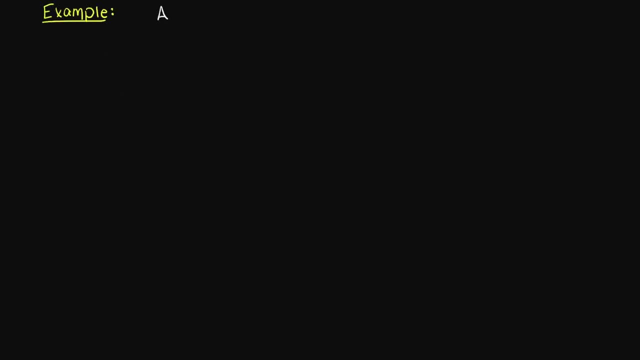 the unknown variables. I recognize this can sound a little daunting. however, let's work through a quick example and you'll see it's not that awful and is actually quite amazing at saving us time and work. So let's take the following matrix and solve it using LU factorization. 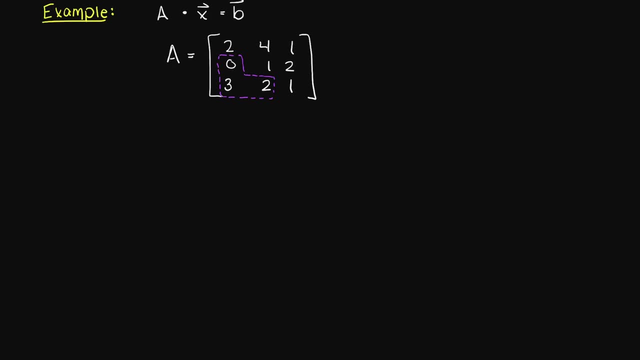 So we must find our U and L triangles And our new constant vector, which will just be the result of solving for our U matrix. Now let's start solving the problem Like we did Gauss elimination. we must turn all the values in the purple triangle to zero. 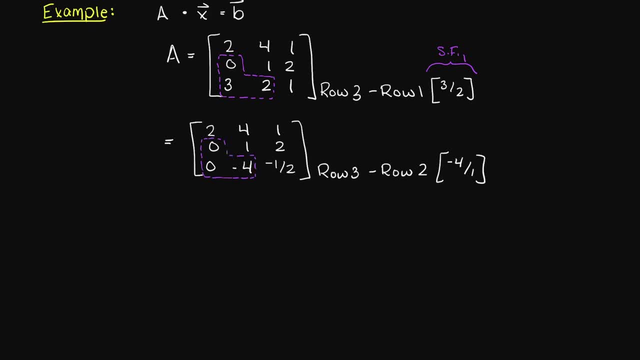 This will result in our U matrix. once completed, We perform the following formula: for each of these three elements that we must turn to zero, And for every element that we turn to zero, we take the scaling factor and plug it into the corresponding element position in our L matrix. 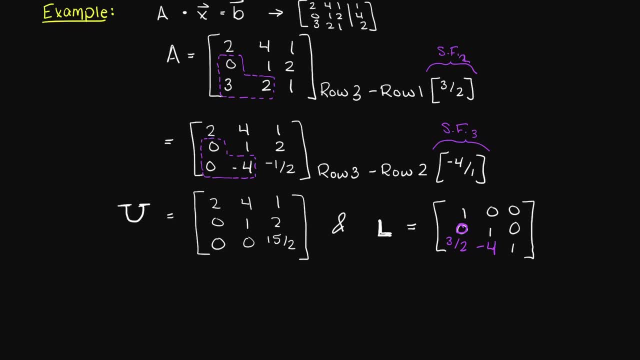 And that is how our L matrix is built. Now we can just repeat this process for the remaining elements. that must become zero. Just be careful with the negatives in your scaling factor, as it can become very easy to make a sign error if you are working too quickly. 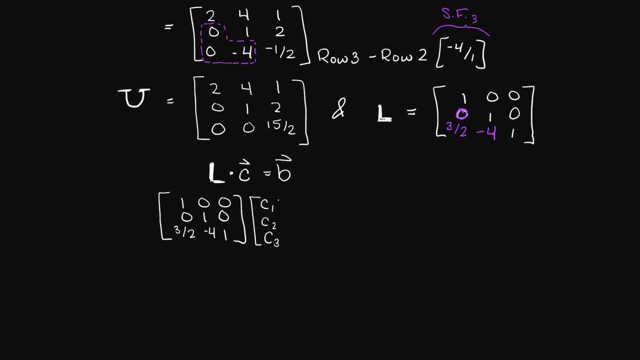 Now that we have our L and U matrices and our new constant vector, we can solve our system. So we take our L matrix times our new constant vector, which equals our original constant vector. Then we simply use forward substitution and solve for our new constant vector. 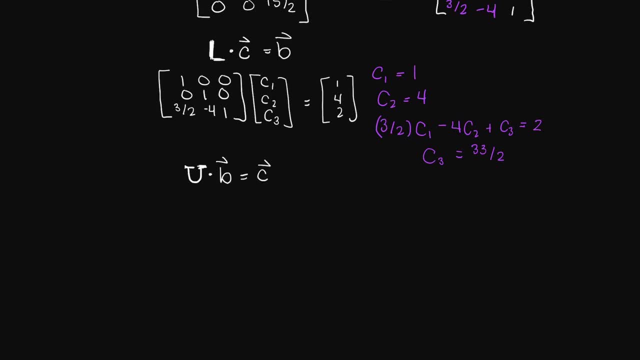 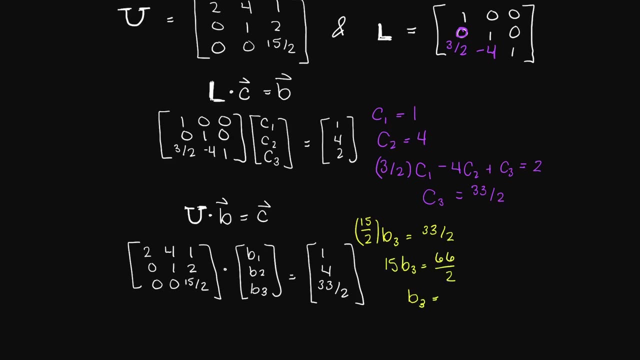 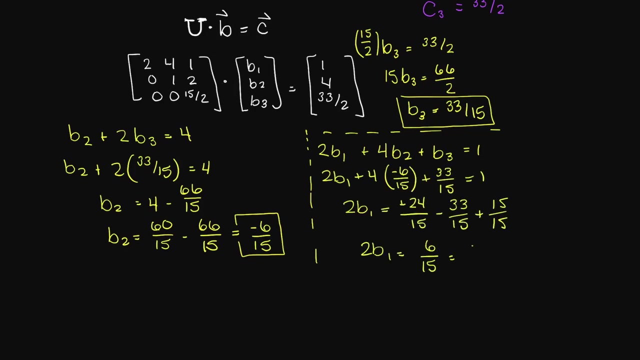 Then we apply this to our U matrix, times our unknown values vector equal to our new constant vector, And solve using backward substitution. And there we go. we have now just solved a system of linear equations using LU factorization. But why do we need this over Gauss elimination, you may ask. 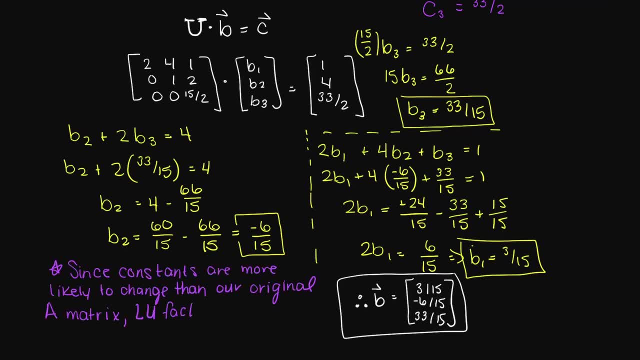 Well, there are several reasons. Typically, the A matrix in a problem is going to stay constant, but the constant values will change more often. Arranging our A matrix into a U matrix: This is the computation heavy portion of solving a gauss elimination problem. 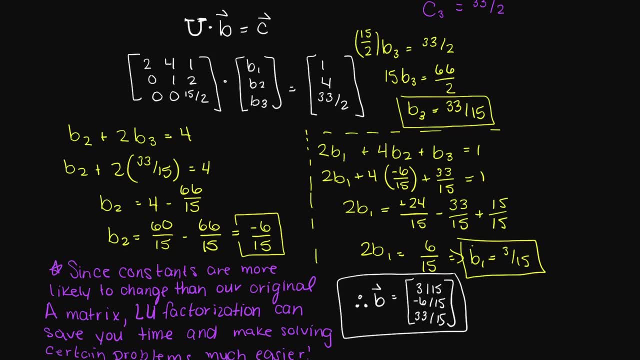 This means it basically takes more calculations and time for our computer or us to solve that portion of the problem. So through using LU decomposition we only need to solve A once and then can apply those values that we find and plug into the L matrix to solve for our constant vector, no matter what. 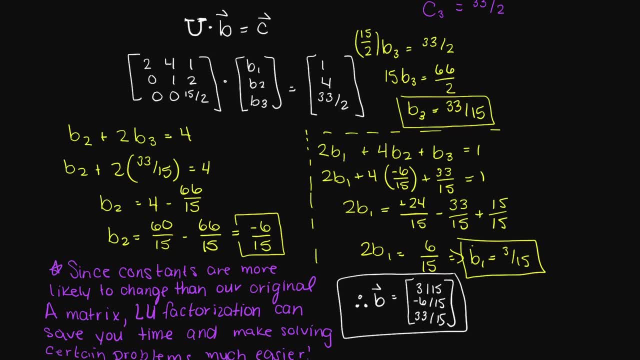 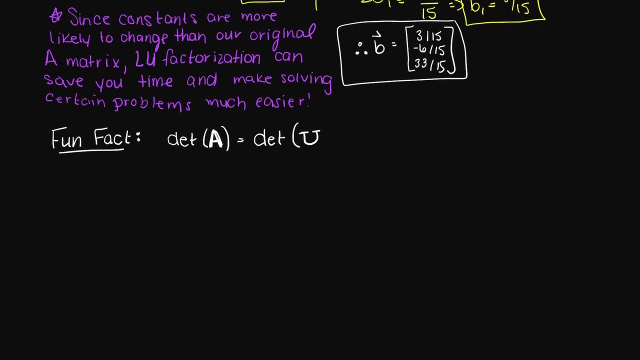 the values are. This saves our computer lots of work and makes our programs much, much easier. Also, if we wanted to calculate the determinant of A, it is simply going to be the determinant of U times, the determinant of L And, if you remember, the determinant of any special matrix. 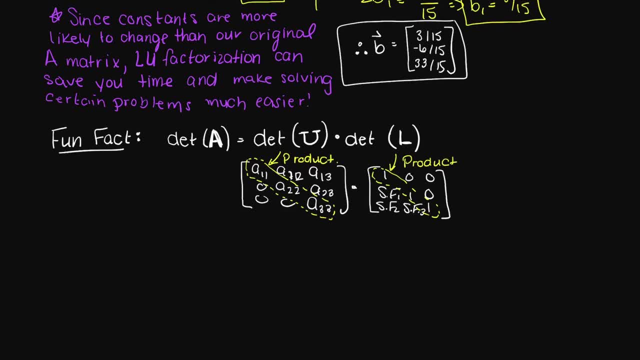 C is just the product of the diagonals. Therefore, finding the determinant of A is also super simple when using LU decomposition. In summary, LU factorization is not much more complicated than gauss elimination and can allow for a simplified matrix solution For whatever values we could enter into our constant matrix.